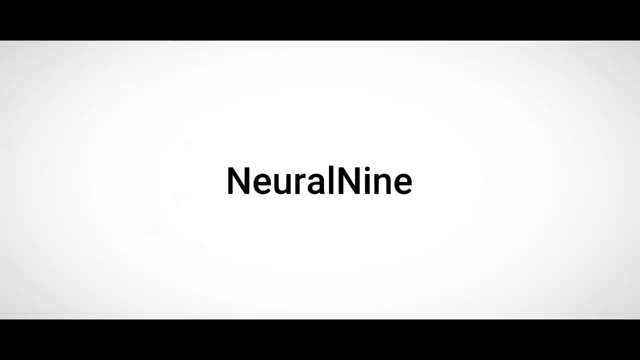 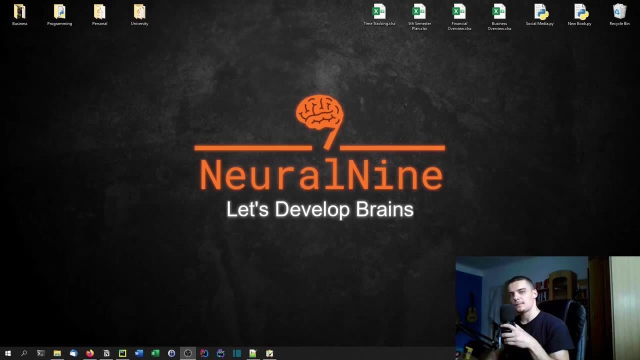 what is going on, guys? welcome back. in today's video, we're going to implement linear regression from scratch in python. and a warning right ahead: it's gonna be mathematical, so let us get right into it. all right, so let's get started with the very basics of linear regression. what is linear? 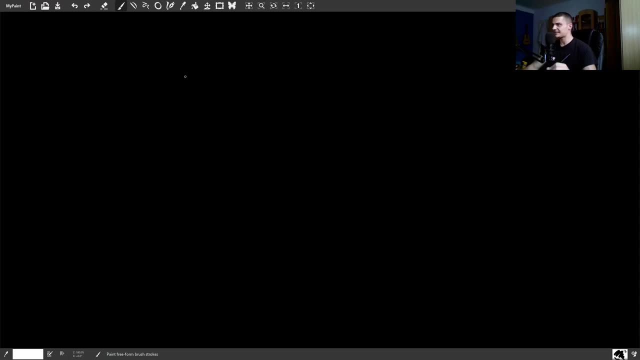 regression and what can it be useful for? and we're going to start with an example right away. let's say we have a bunch of students and these students have an exam and they have a certain study time. each of them has a certain study time that they invested for this exam. so let's say we have the 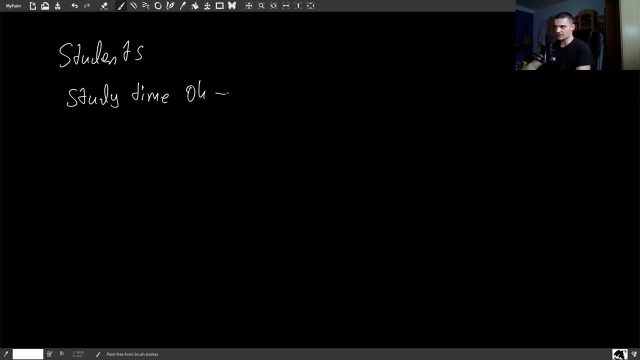 study time. here it can go from zero hours up until not really infinity, but pretty much infinity, depending on what the maximum number is of the students. so you can study two weeks in advance, one year in advance, you can study one minute in advance, from zero up until, let's say, limitless. 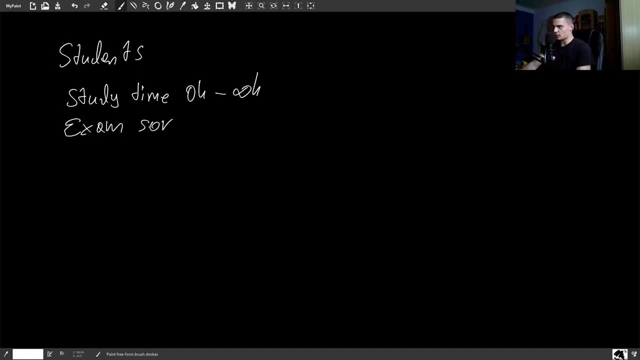 and then we have an exam score, and the exam score is the actual result of the test, and it can go from zero points to 100 points or from zero percent to a hundred percent. so what we can do now is, let's say, we have a data set with 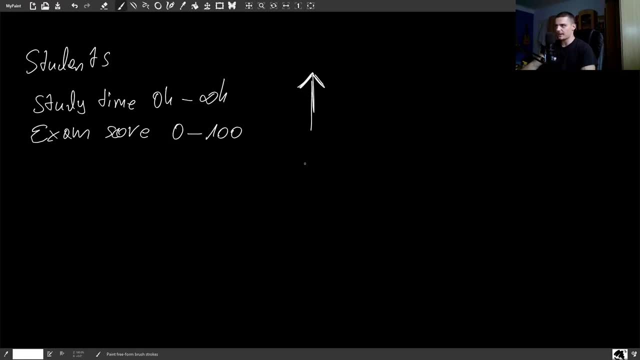 these data points and we want to plot this here on a two-dimensional coordinate system. that's not the most beautiful coordinate system, i know, but let's say the x-axis is the study time and the y-axis is the exam score. now, if we were to visualize all these points, we would probably 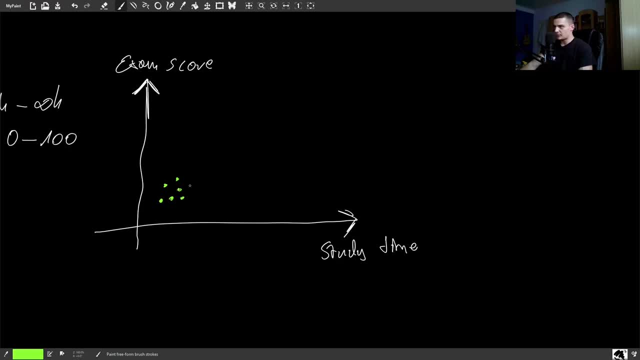 see something like that, with a bunch of data points here: people who don't study at all and get pretty low scores. people who study a little bit get better scores, but still some that get pretty bad scores and all that um, and we can see all these data points, people that study a lot- and 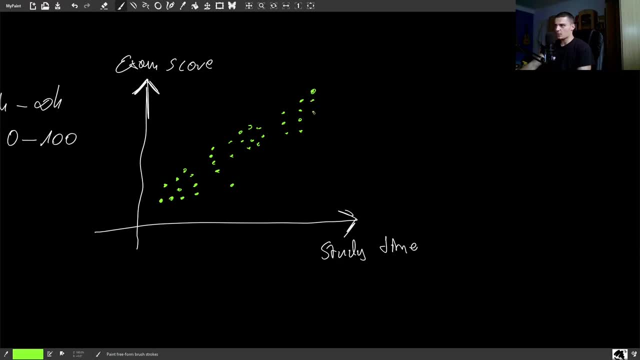 get a lot of uh points or a very high score, then some people who study a lot and don't get very good grades at all, some people who don't study at all and get very good- uh good grades. those are the outliers, but most of the points are going to be somewhere here in the middle now with linear. 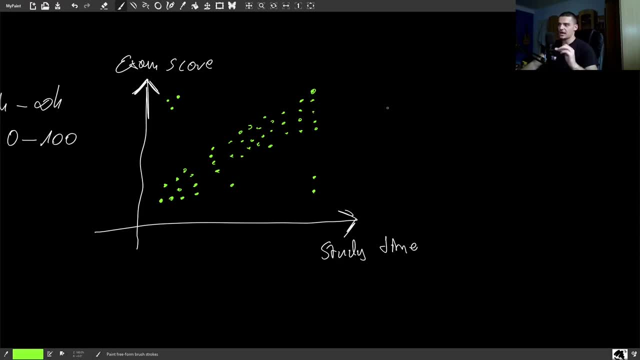 regression tries to do? is it tries tries to find a line that fits these points the best. now, best is a little bit subjective, because certain regression types or certain algorithms use different, uh, approaches, because some say: okay, i don't care about outliers, i care a lot about. 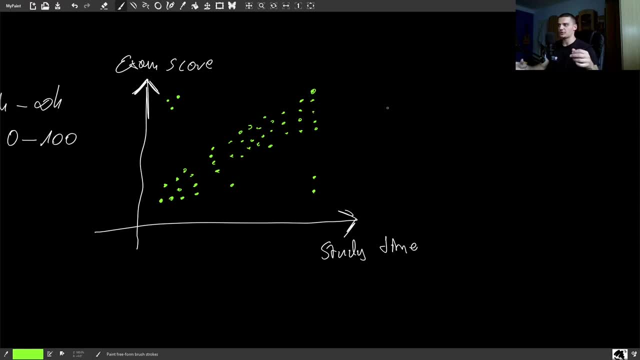 outliers and so on. depending on what you want, you have to choose a different procedure. but for linear regression, what we're interested in is minimizing the error, and the error is basically, let's say, i have a linear function here, a blue line like that, and this is obviously not the best. 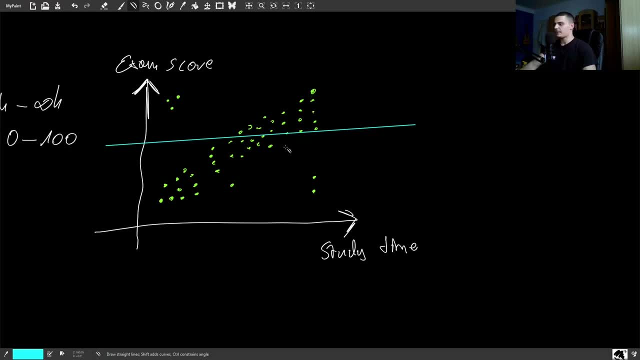 function that we can find for this, for these data points. but the error of that function would be to basically go for each point and see if this function was correct. we would predict that for this x value here, this would be the y value, and then what we do is we just go down and see. okay. 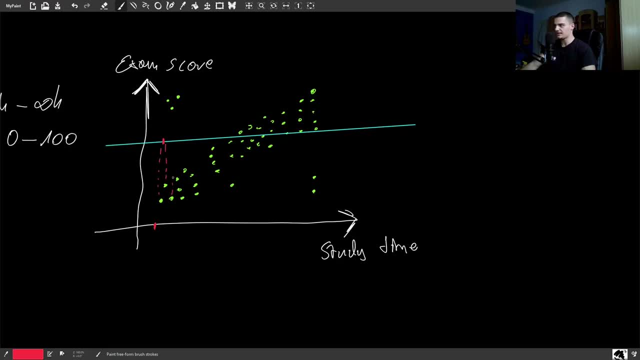 this here is the error, and this here is the error, and this here is the error. this is just a difference from the prediction to the actual reality. that is the error. okay, and what we want to do is we want to find a function that minimizes that error, and this is what linear regression is about. so the structure of a function. 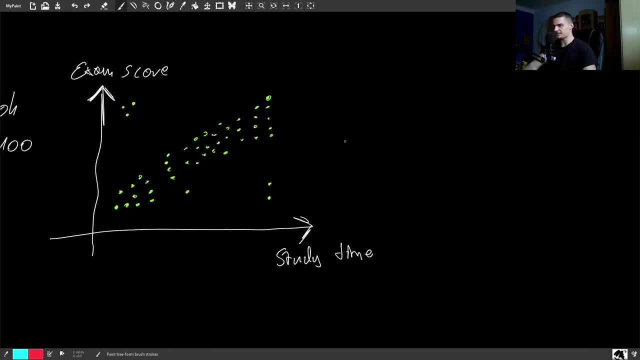 is basically of a linear function is basically: y equals m times x plus b. so m is basically the steepness and b is the distance here. so we expect the line, the final line, to be something like that. if we tolerant this to be, maybe it's more like aлет to the z. i'm just gonna try toนะ. 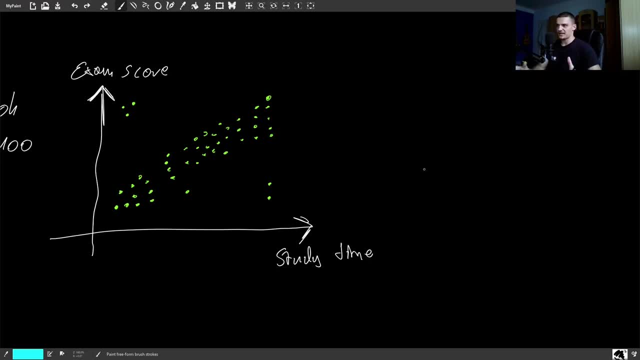 scheme, do what you just saw. uh, take this, keep this six, five, five and so forth here. so we're gonna set this up and then we're gonna go down there and and we're gonna do this in this selected way method about in a second. but in order to minimize something, it has to be something that produces. 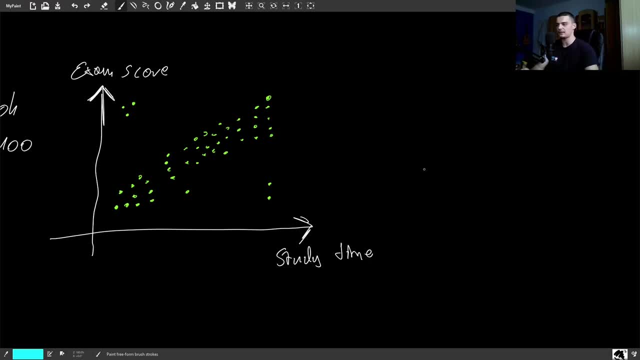 a value because we want to minimize the output by tweaking the little things that we can't tweak. in our case, if we look at m times x plus b, we want to manipulate, we want to tweak m and b so that for x i get the best possible y with the least error, and the error function needs to be defined. 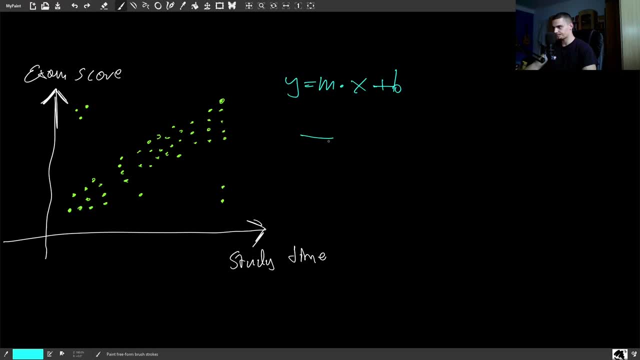 in order to minimize it. so the error function is going to be e capital. e is going to be one divided by n, which is. i'm going to to tell you in a minute, because in a second, why it's one divided by n times the sum from i equals zero up until n, and now we get y, i, which is the actual. 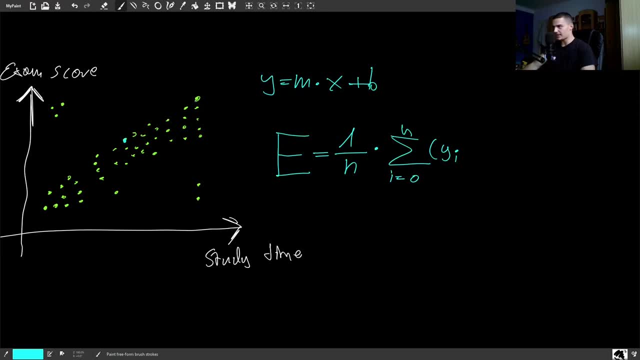 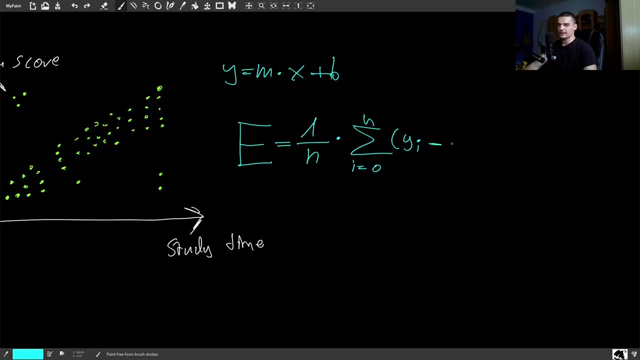 value that we get here. so this point is y i and this point is y i. the value, the y value of this point is the actual y i value and from this we subtract y i, uh hat, for example. so this is just the the predicted value. this is this value here, and we can actually remove that and replace it by. 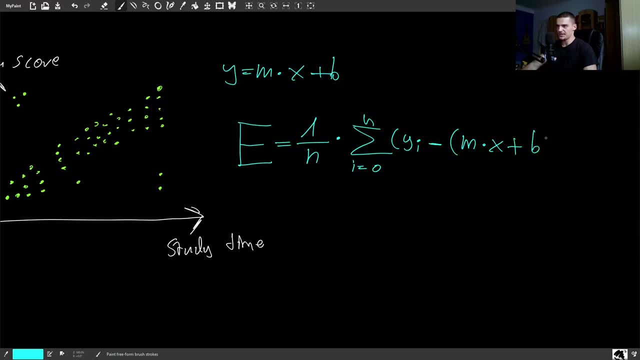 m times x plus b. so that is the error and we can square that and that would be the mean squared error, and we can add an i here to make it a little bit more accurate. so if you have never seen this before, this is called the mean squared error function. 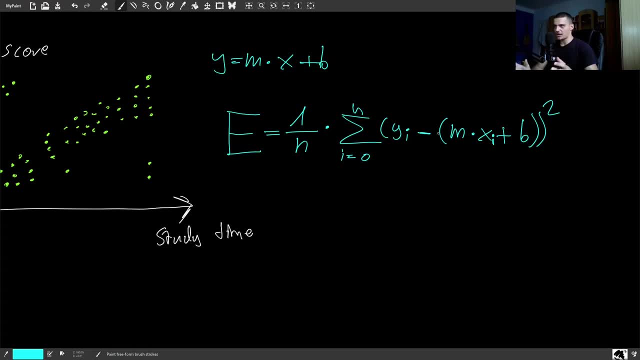 don't be confused, it's not really complicated. it may look complicated because it's math, and for a lot of people math looks just complicated. but all we're doing here is this is a mathematical way of writing that for each point, and n is the amount of points for each point from zero, from the zeroth. 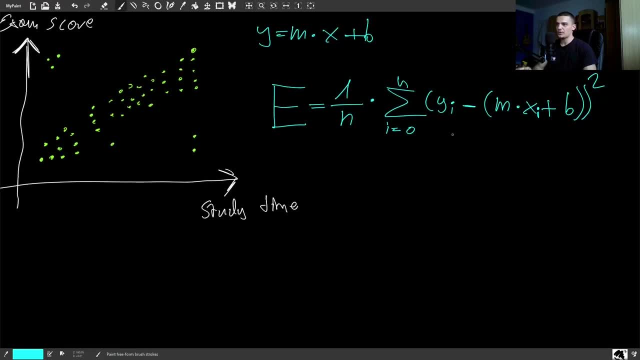 point. from the first point to the last point. what we do is we get the y value of the actual point, so this y value here, or this y value here, and we get the y value of the actual point. and we get, or this y value here, the actual value, and we subtract um the position of the function y value. 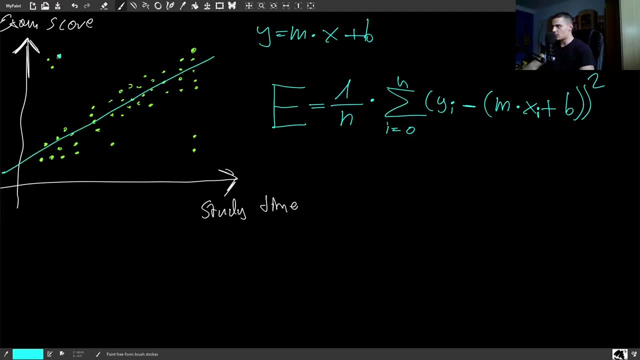 so if we have a function like this, we will take the actual y value here and this y value here, and this is the difference. so this is what we're going to get, and then we square that difference and in the end, we take all these distances, all these errors that we have, and we divide them by 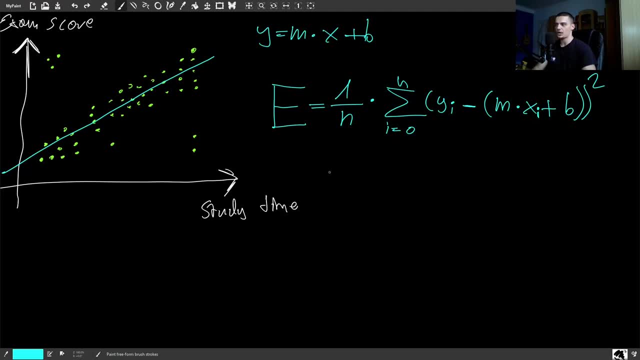 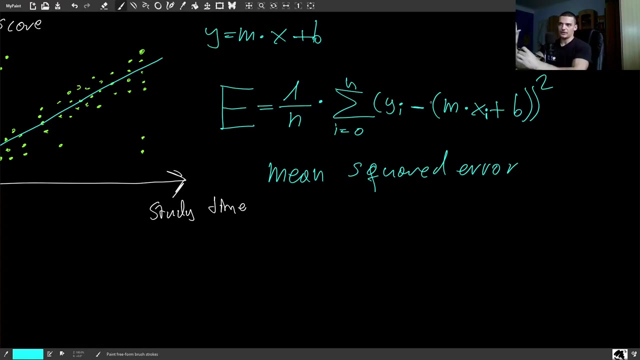 n, which is the amount of points. so we get the mean squared error. so this is what this function does. it's just a fancy way of saying: take the difference from all the actual points and what the function would predict. the proper y value would be square. that. 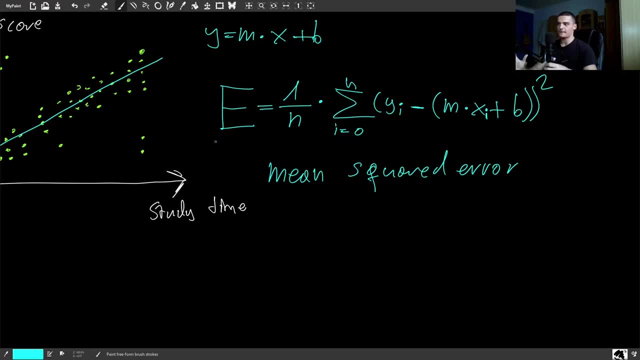 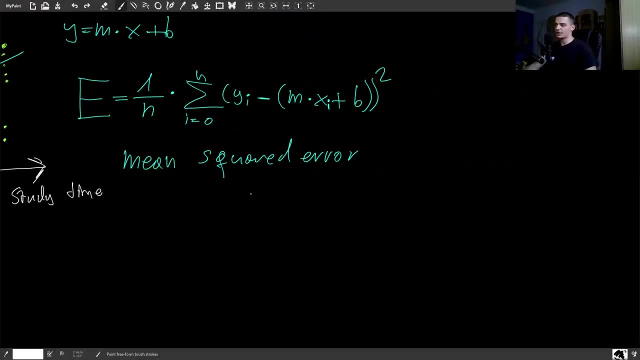 difference and divide it by the amount of points that we have to get the mean squared error. this is the error function that we're trying to minimize when it comes to linear regression. all right, so this next part here is going to be very technical and mathematical, because we're going to talk about partial derivatives, about calculus. 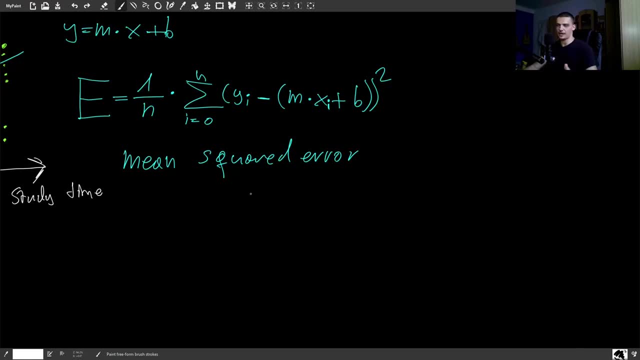 so if you're not interested in that, or if you don't understand calculus at all, you can skip to the coding part directly. uh, i would not recommend it, because even if you don't understand everything, it's good to just understand or listen to what is happening behind. 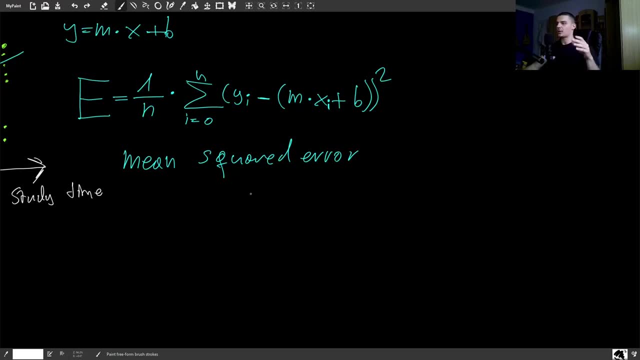 the scenes, even if you don't understand all of the math, um. so i would recommend you to watch that part as well, but it may be a little bit boring because it's very technical and mathematical. i personally think it's one of the most exciting things: to understand what is. 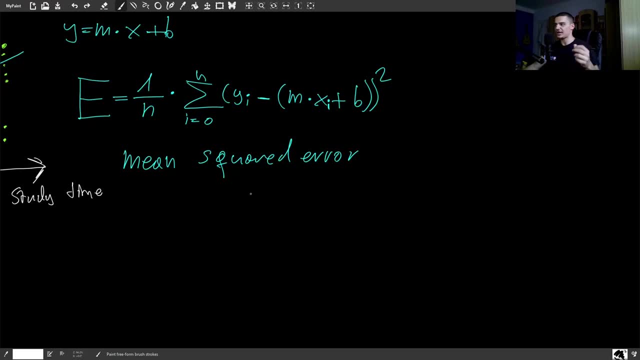 exactly happening? how does this optimization work? but i can understand if some of you guys say i don't want to listen to that, i want to get to the coding. just keep in mind that you won't understand fully what is happening behind the scenes, so let's get into it. um, we want to minimize that. 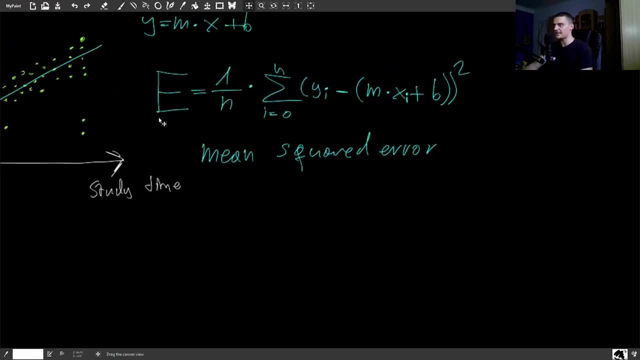 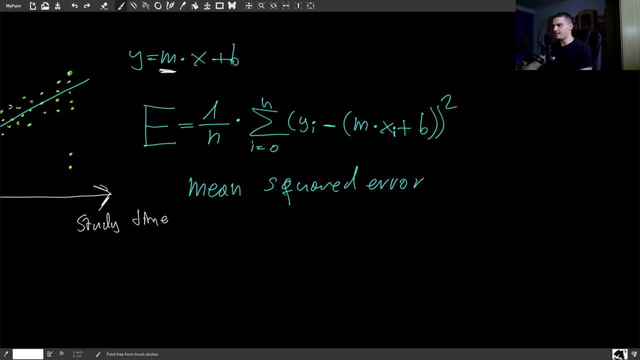 error function. we want to get the lowest possible e for our line. we want to find the line that gives us the lowest possible e. so the only thing that we can influence is the m and the b. the x is just the input and the y is just the output. 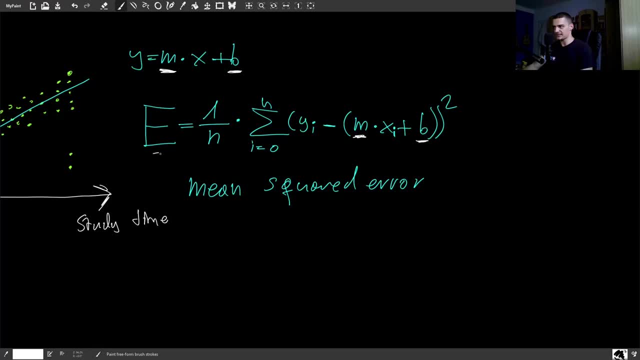 we want to find m and b so that we can minimize e. that is our goal. and how can we do that? we can do that by taking the partial derivative with respect to m and with respect to b, because that gives us the direction of the steepest ascent with respect to m and b. so how can we change m? 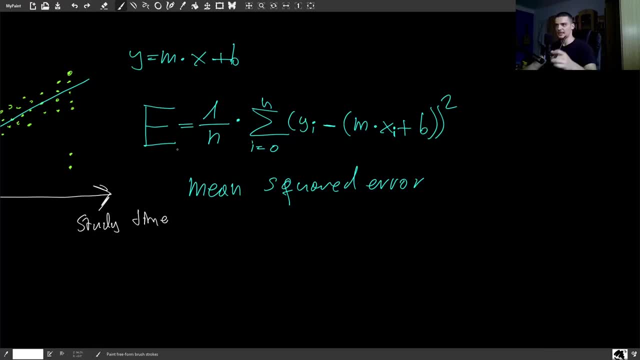 to maximally increase e. and how can we change b to maximally increase e? now you might say, okay, didn't we want to decrease e? yes, we did want to decrease e, but if you just take the opposite direction, if you have the direction of the steepest ascent, you can just go the opposite direction and you have the 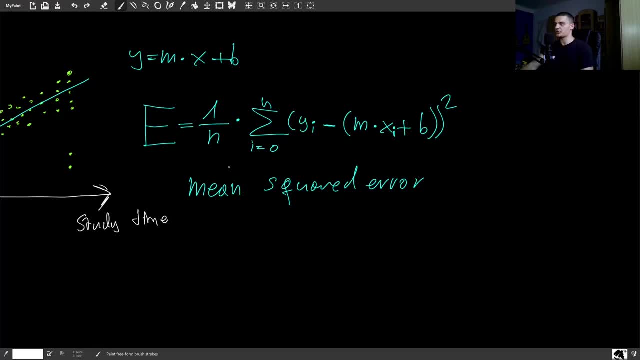 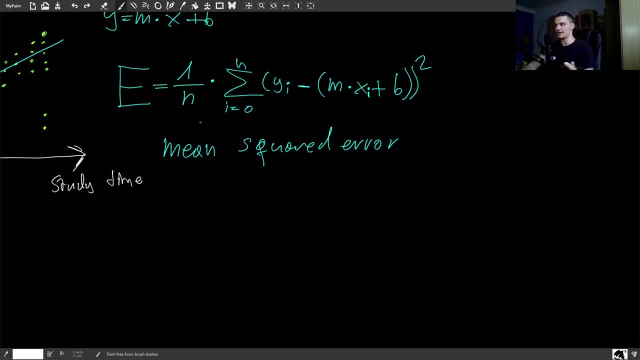 direction of the steepest descent. so this is what we're going to do: we're going to take the partial derivative with respect to m and b and then we're just going to go to the opposite direction of this gradient. so we're going to say the partial derivative of e with respect to m is going to be. 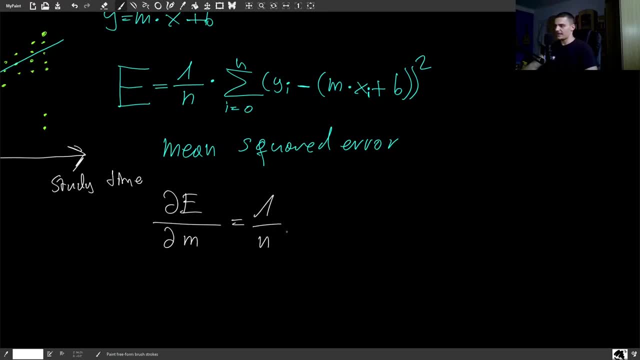 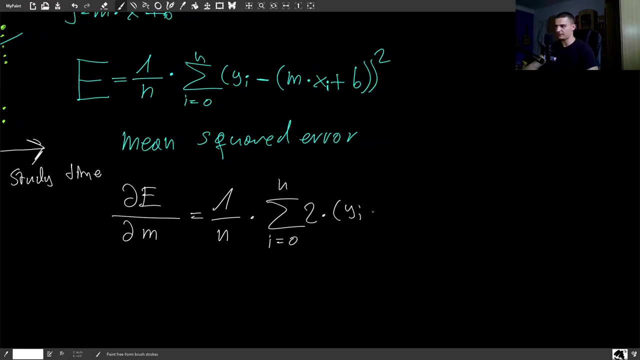 or is actually one divided by n times i equals zero to n. and now we have this squared here. so we say two times. those are just a basic calculus rule. so if you don't know calculus, don't be confused, you don't need to understand everything. minus m times x, i plus b, and now we need to also multiply with the. 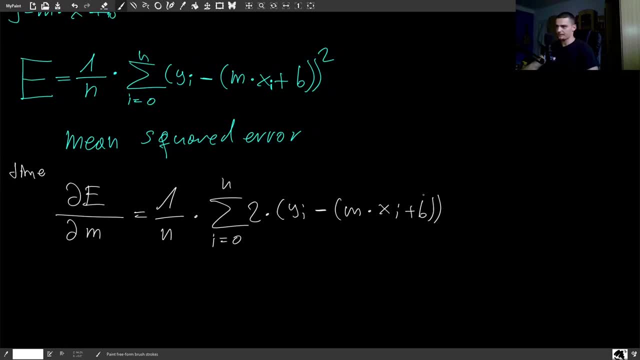 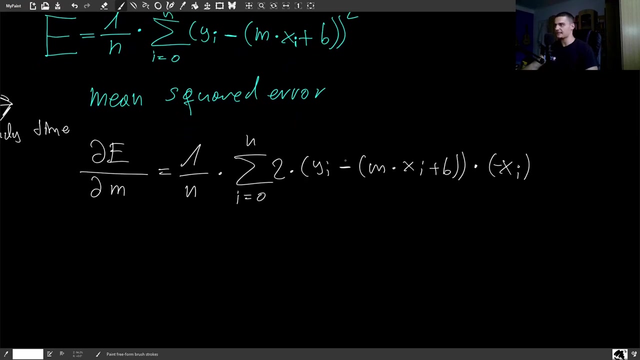 inside derivative, which is basically just: this is a sum, so we just ignore it, and this is the factor. so what we end up with is negative, x, i, um. and now we can simplify that by just extracting the two and the negative. so we can say: okay, this is nothing but just minus two divided by 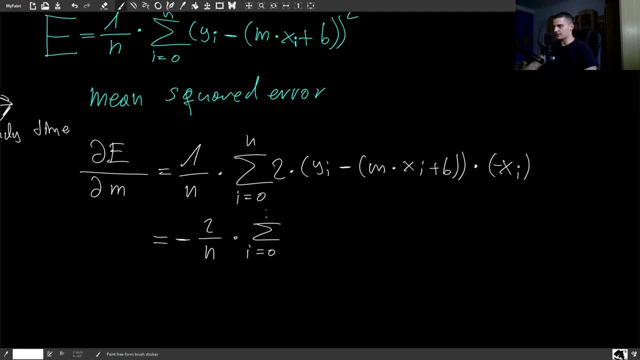 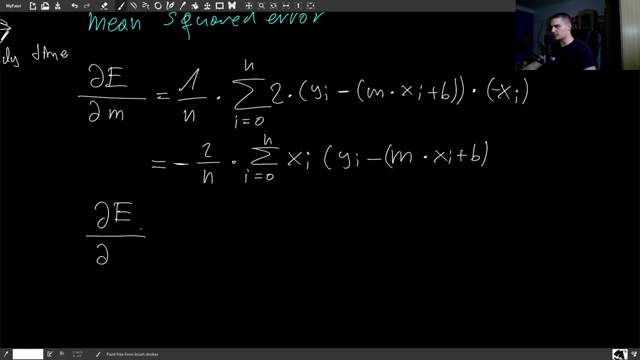 n times the sum from i equals zero up until n, and then we have x? i times y i minus m times x i plus b. so that is the partial derivative with respect to m. now let's do the same thing for b. it's basically the same, but the difference is that we don't have the x- i, because here we don't. 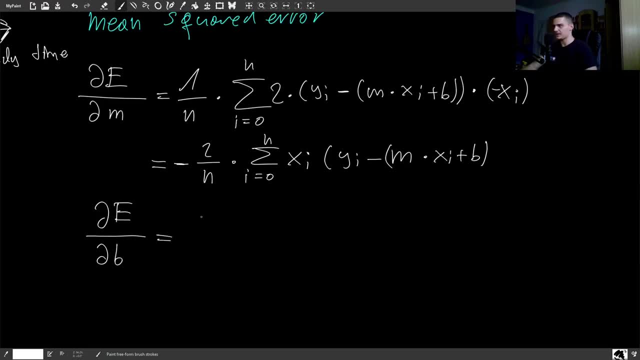 have a factor, so this is actually the same thing. um, we basically have negative two divided by n times sum from i to n, and then just y i minus m times x, i plus b. that is it and this. those two things give us the direction of the. 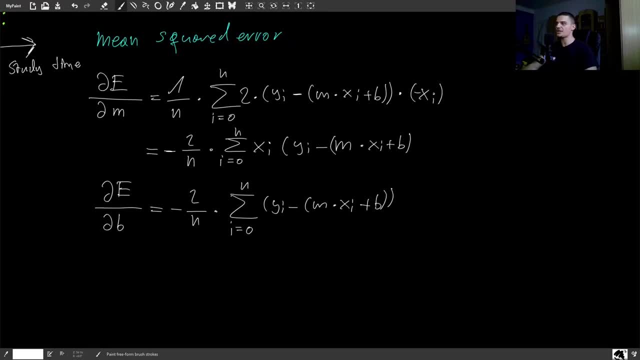 steepest ascent with respect to m and b, and all we need to do now is we need to go to the opposite direction. that's all we need to do. so if we want to improve m and b, all we need to do is, with each iteration, we say: take the current m, and what you do is you assign to it. 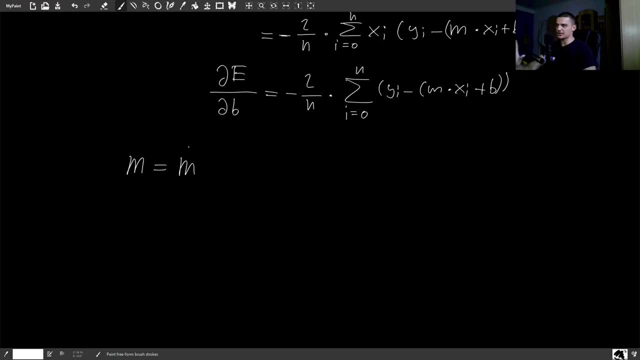 the current or take the new m. what you do is you assign to it the current m minus a learning rate- we're going to talk about that in a second times- the direction of the steepest ascent. so, uh, basically, e and m and the same for b. b equals b minus l. this is more of a programming notation. 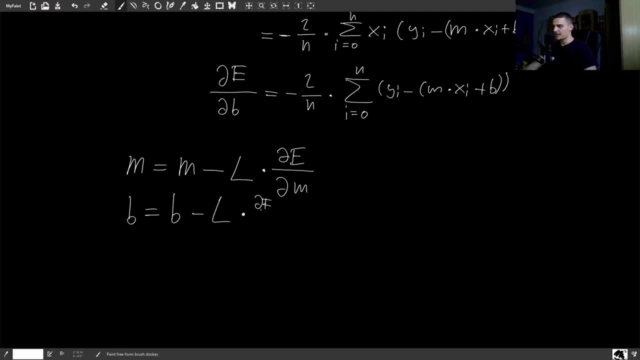 not necessarily a mathematical notation, but that is the direction of the steepest ascent, what we do, so we know, okay, in this direction let's say, uh, we increase the error the most. so what we do is we just go the opposite direction, and we do that with each iteration because it 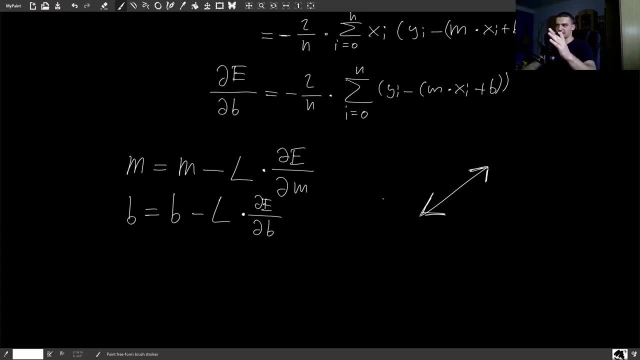 changes right. so sometimes in this direction it's going to be the steepest ascent. uh, then in another direction, then again in another direction, especially if we don't just deal with two variables but with many different variables. we don't do this only with uh score and with um study. 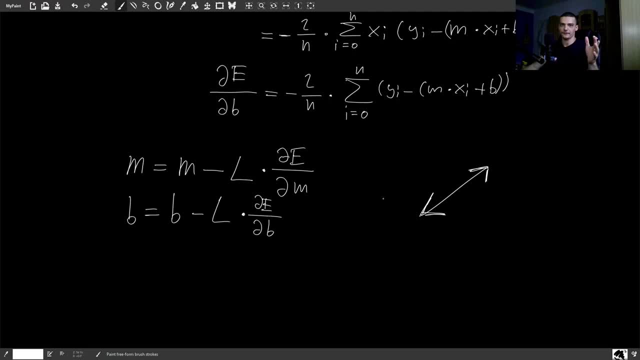 time. sometimes we have like 10, 20, a thousand different features that we have to take into account when doing a linear regression, so it's not always just two things: um and this again, this is the direction of the steepest ascent, which is why we subtract, because we don't want to go to. 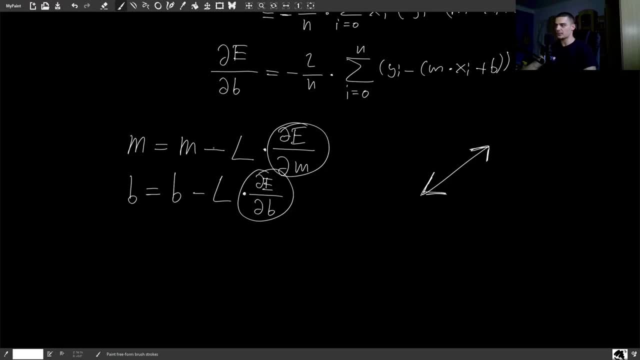 that direction. we want to go to the opposite of that direction, otherwise we would have a plus here, not a minus, and the learning rate is basically: how big, uh, how, how large are the steps that we take? now, the larger the steps, the faster we're going to get to the steepest ascent. 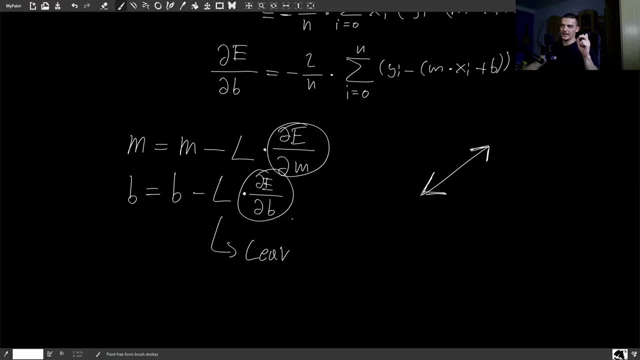 we're going to get to the actual optimization, but the lower the learning rate, the better it's going to be in the end, the the better the result is going to be, because- because we're paying attention to details much more, so i think we're going to go with a learning rate of about 0.001. 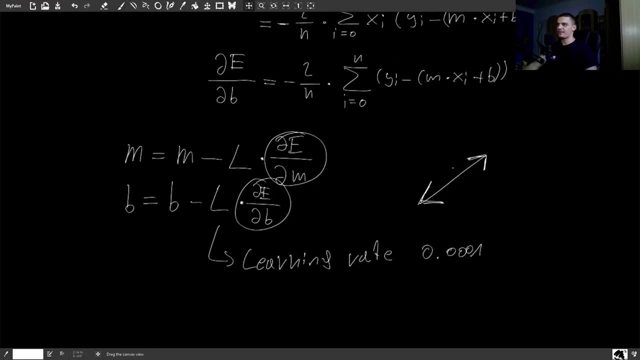 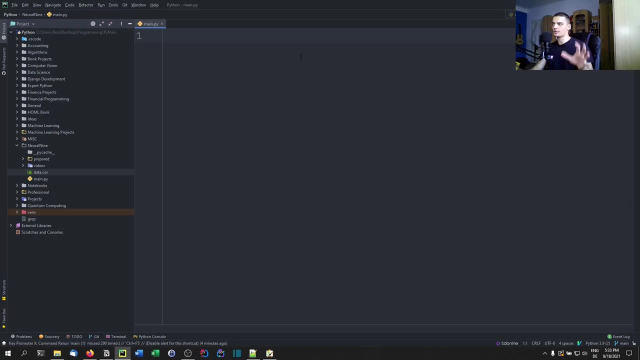 which is, or maybe one more zero. um, we're going to do that, and now that we have all the math handled, we're going to do this in python. now we're going to take all this theory and turn it into python code, and for this we're going to start by installing two libraries. however, since we're 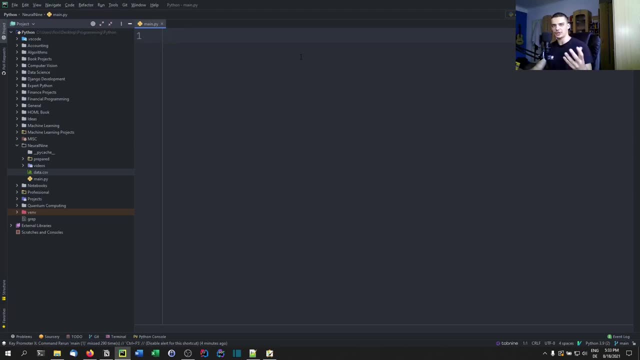 implementing linear regression from scratch. those two libraries are not going to be related to the linear regression algorithm. we're just going to use pandas to load a data set from a csv file and we're going to use matplotlib for visualization. the whole linear regression process will be. 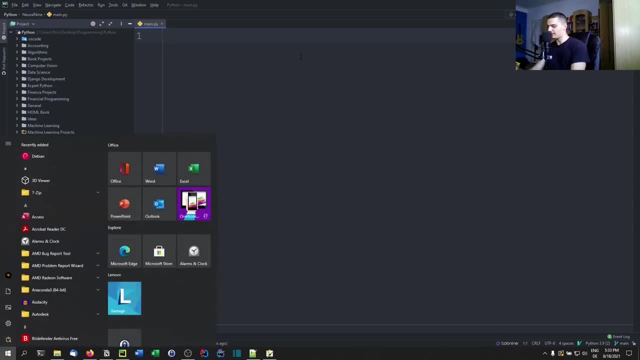 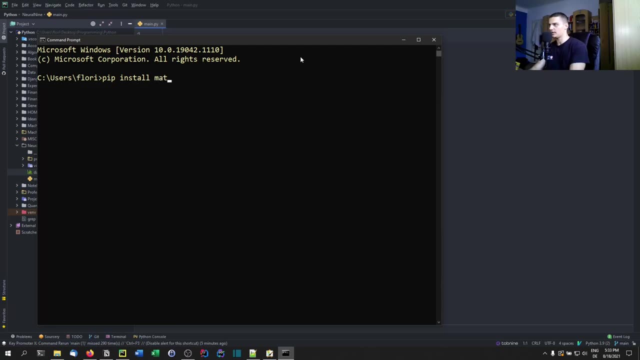 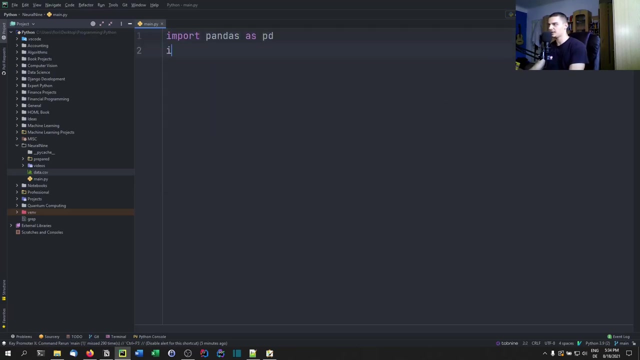 implemented by us from scratch. but if you don't have pandas and matplotlib, you want to go to cmd and say: pip install pandas and pip install matplotlib. like that, and once you have that, you can just go ahead and say: import pandas, spd and import matplotlibpiplot as plt. now what you're going to need is some sort of data set. 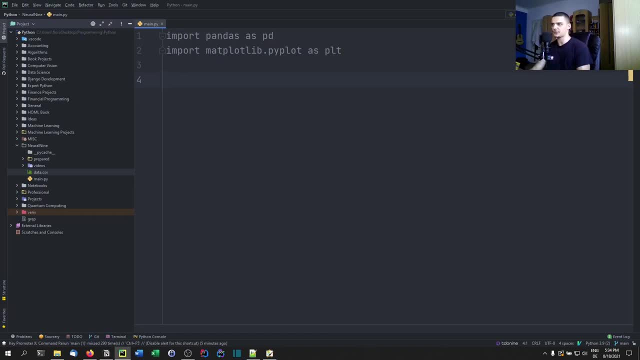 you can craft your own. you can just make up some values, or you can, if you're comfortable with that, take an actual data set and apply linear regression onto it. for this video, i have just crafted my own sample csv file, just some random values that have a certain trend inside of them. 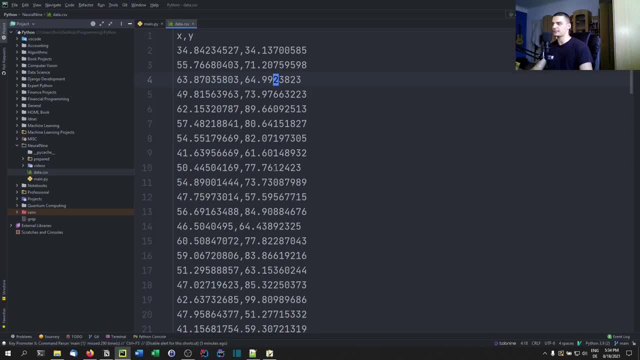 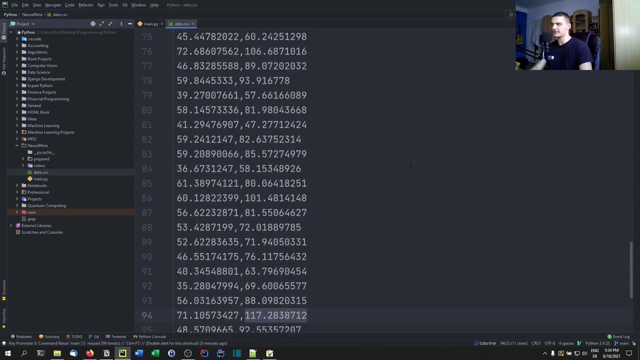 we have x, y and then just a bunch of random values here, randomly generated, however you can. you can, as i said, go with a real data set and we can also interpret those as study time and score, if you want to. however, i think we have some values above 100, as you can see here. 117. 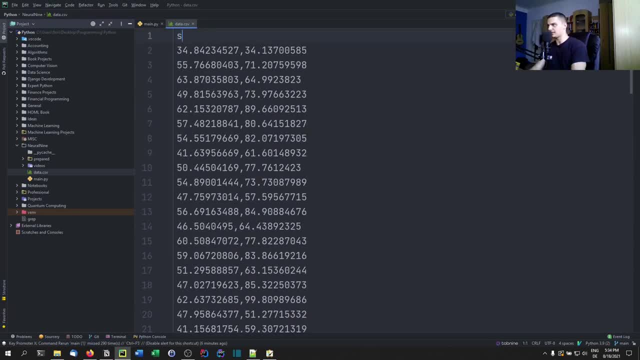 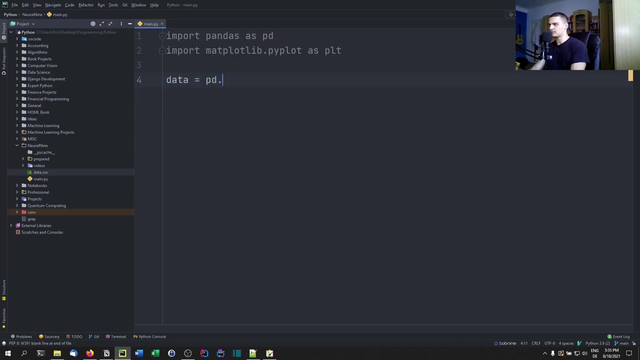 so it's not entirely accurate, but we can just go ahead and call this study time and score. so this is just a basic comma separated value file, csv file with some random values. we can load them in by saying data equals pd, dot. read csv, data, dot, csv. and then we can take a look at it by saying print data to see the structure of the data. 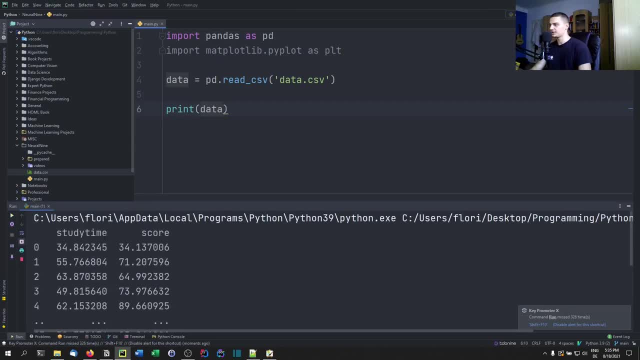 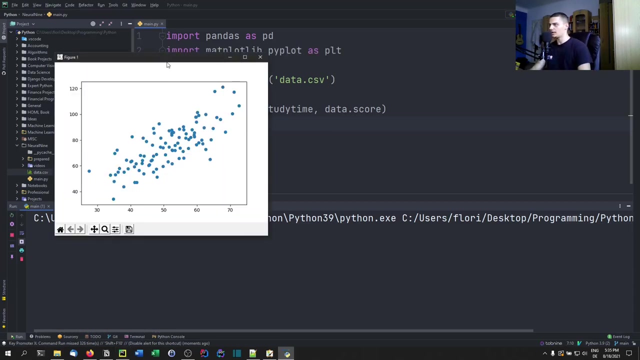 frame. nothing too fancy. two columns, study time, score and the values. we can also go ahead and visualize them by saying plt- scatter, data dot- um, what was it? study time and data dot score, and then plt- dot show like that. and there you go. so those are the data points that we're going to use for this regression example. 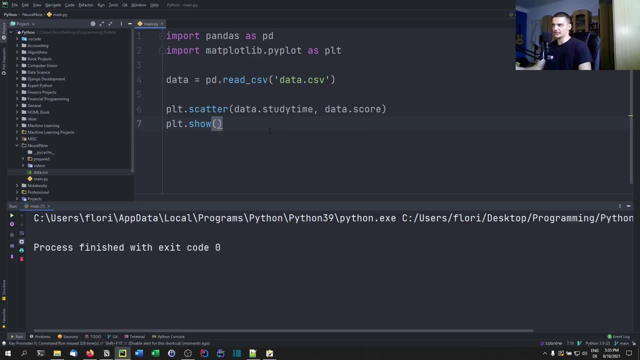 here you can actually pick any data points. the data is not the focus here, we just want to have a properly working algorithm. uh, so i'm going to delete the visualization here and we're going to start with the loss function. so we're going to say def loss function. you can also call this mean. 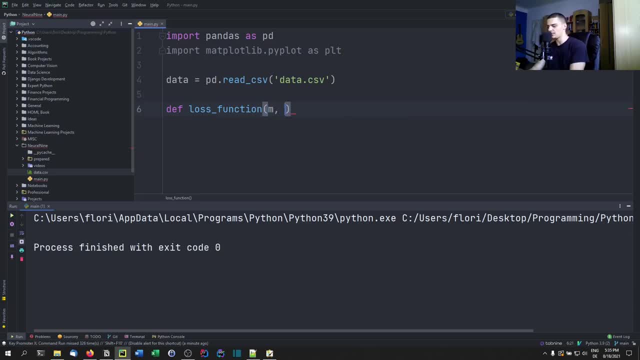 squared error. and to this function we need to pass the msql function to the data function. so we're going to say m value, the b value and the points that we have, the actual data points. so in our case, data um. and what we're going to do here is we're basically going to say we have 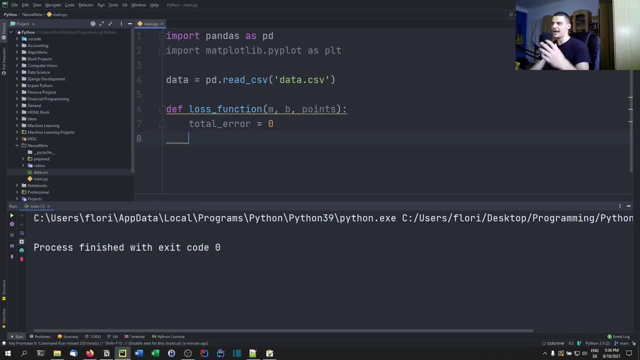 a total error which starts at zero, and what we do is we add all the individual squared errors to that and in the end we divide by the amount of points. so we say: for i in range length and uh, what was it? points we're going to say. 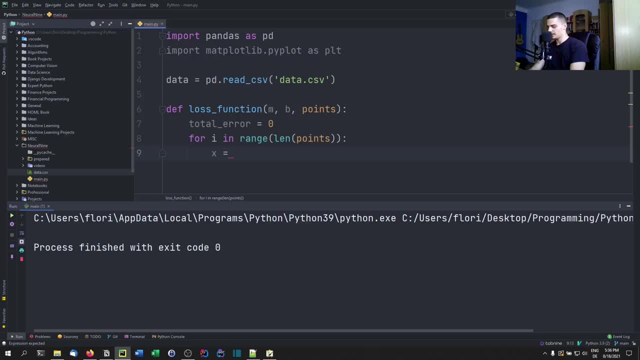 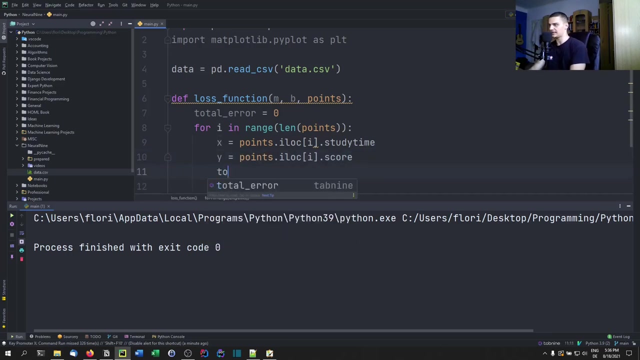 um, the x value that we have is the points dot ilog. so at the location i, we want to have the study time as the x value, and then at the location i, we want to have the score as the y value, and the error is basically just what we had already. so if we look at my paint here, uh, what was the error? 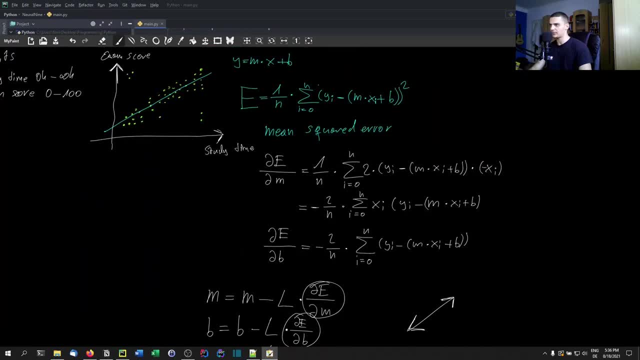 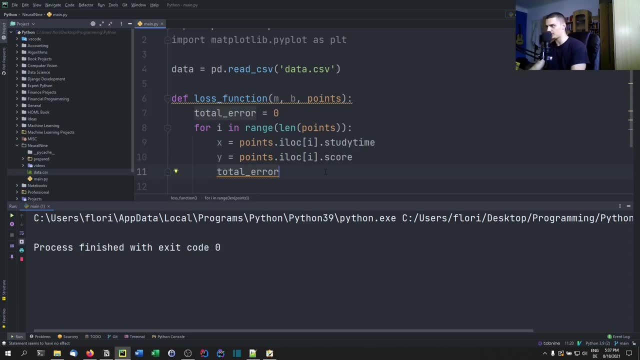 function. there you go here. this is the error function. we're just gonna write it in a pythonic way now. um, so, total error. let me just see how i wrote it. total error plus equals, and then, uh, the loop is basically the sum, and what we write in here is the iteration of this. 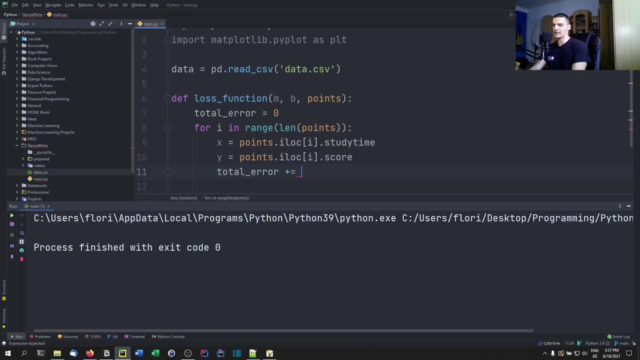 sum uh, sigma symbol. so we say to the total error we want to add y, the actual y point minus what we thought them. y points should be based on m and b, so m times x plus b and the whole thing squared because it's the mean squared error. 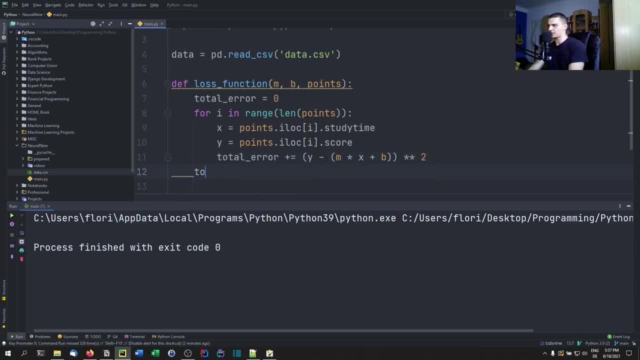 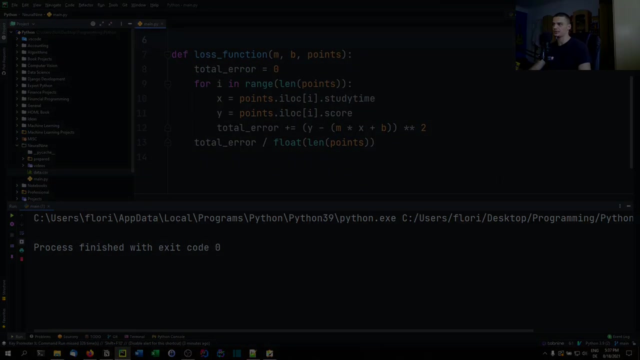 and in the end, what we do is we just say total error divided by float length of points, like that. so that is the basic loss function. it tells us how off, how much we're off, from the actual result. now, what you need to know about this loss function here is that we're actually not going to use it. 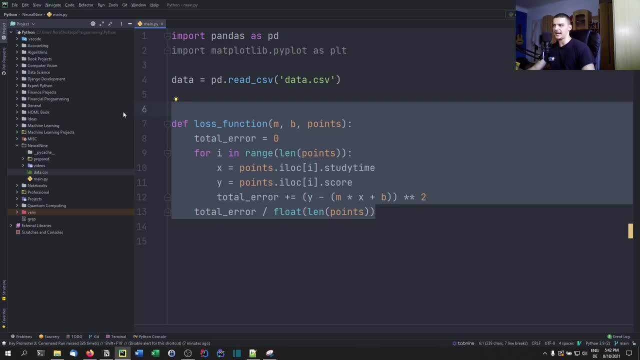 because what we're actually interested in is just minimizing it and it's already included- gradient descent- because we cannot just have this function and tell python, take the derivative of it, so we need to do it manually, and we have done it manually already, so this function is more like 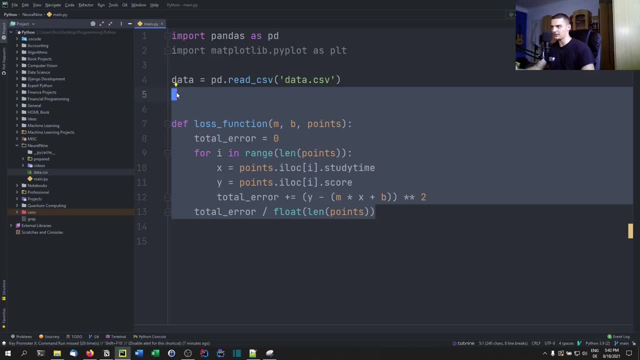 a function that you can use if you want to calculate the loss manually, but we're actually not going to use it in the final optimization process. so let's go ahead and implement the gradient descent. we're going to call this function gradient descent. we're going to pass here m now. 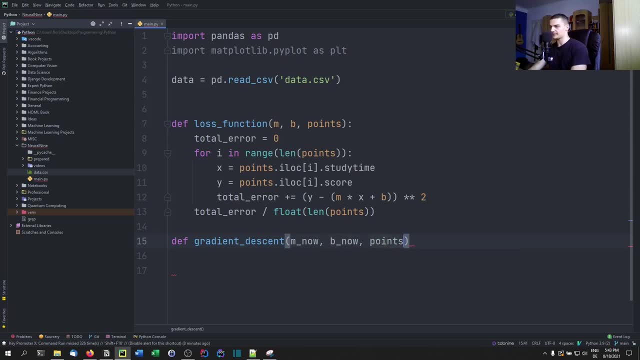 b, now the current values. here we're going to pass the points and want to pass a learning rate l, and what we're going to do now is we're basically going to just start with a gradient for m of zero and for b as well, and then we're going to say n is just a length of the points, the amount of points. 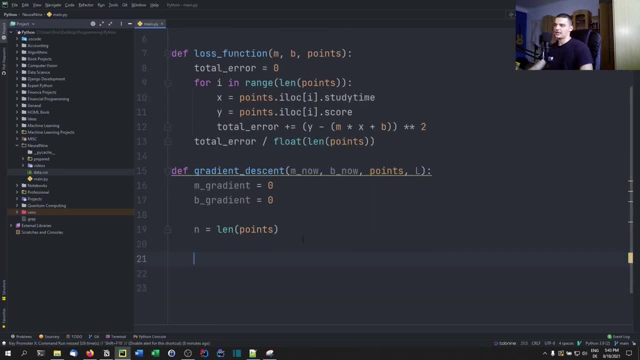 and what we're going to do now is we're going to just perform the gradient descent again. we're not going to use that function. this is just a separate function that you can use manually. here we're going to already use the, the formulas that we had here. so those two formulas here. 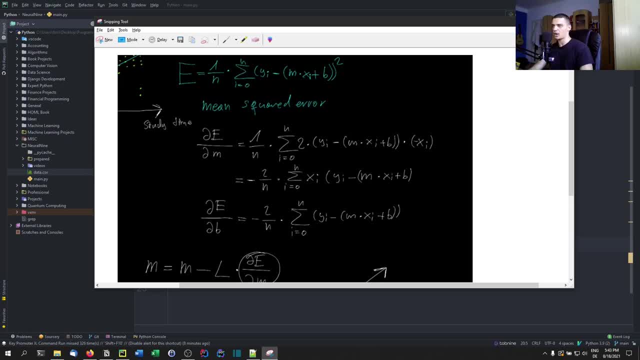 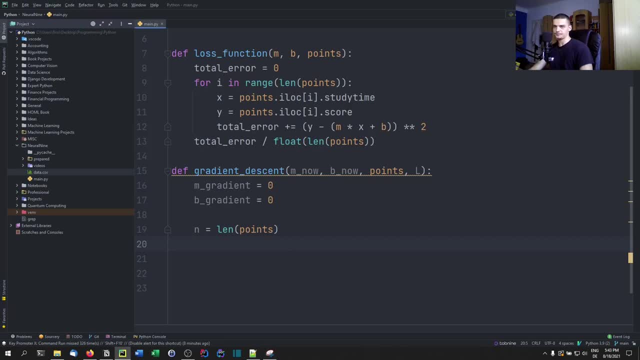 that we already talked about these partial derivatives and those already include the loss function to some degree. so what we're going to do now is we're going to say for i in range n, so for each point we're going to do is we're going to take that point, so x equals then points. 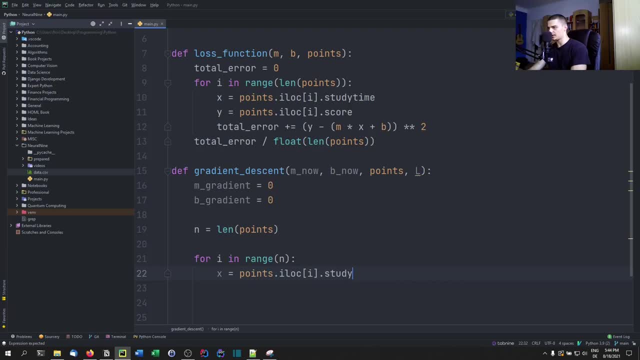 then we taking the linking curve two and the latex angle, so we're taking theước again, crossing out the2000 and doing a solidategical operation, and then we're going to calculate how much the gradient should be. so we're going to say we're going to calculate y, i maybe 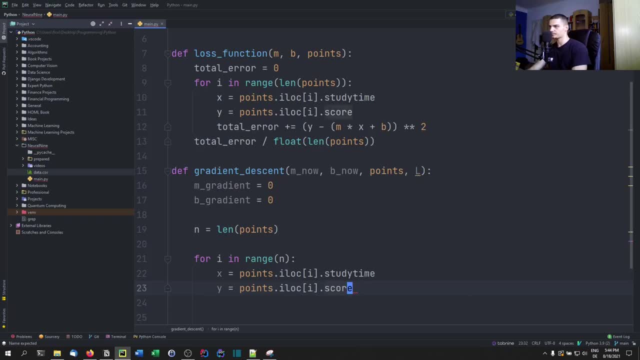 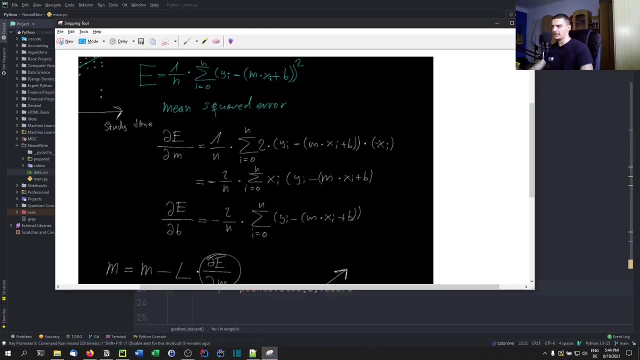 take the gradient of the value from 5 to 10, and then we're taking the gradient for years. so we're going to say, for m i, how about dot i in there? and then we're going to welcome this point along the delta so that we just자가 one point and we're going to y equals. i log istudytime. 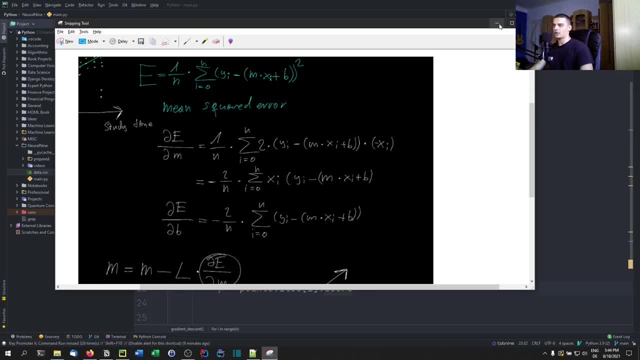 and then y equals ilog iscore, and what we're going to do now is we calculate the gradient based the loop is the sum symbol here. All I'm doing here is just putting this into Python code. If you want to understand what's happening here, you need to go back to the mathematical explanation. 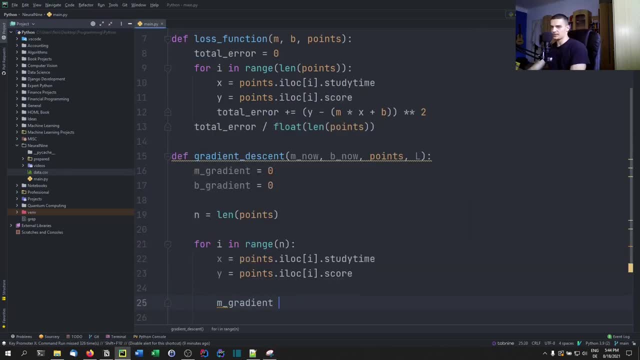 So we're just going to say m gradient plus equals, and then negative two divided by n. actually the negative is out here. negative two divided by n. times x. times y minus m at this particular moment in time. times x plus b at this moment in time. 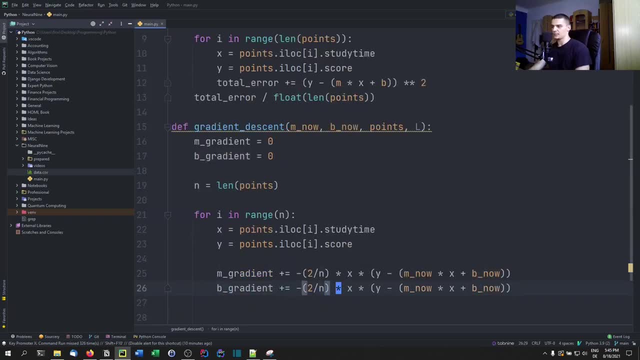 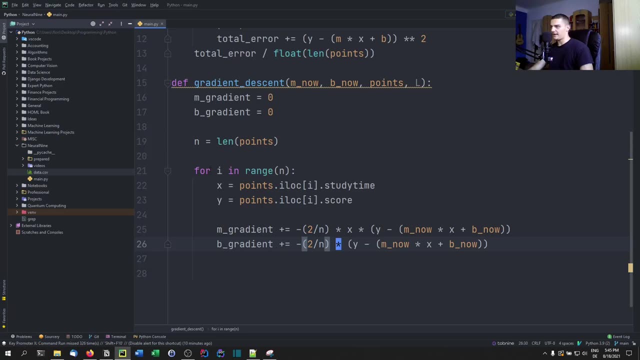 and then b is basically the same, but without the x. There you go. Then, once we have that, once these iterations are done, we know which direction we have to move into or away from actually. So we're just going to go back to the mathematical explanation. 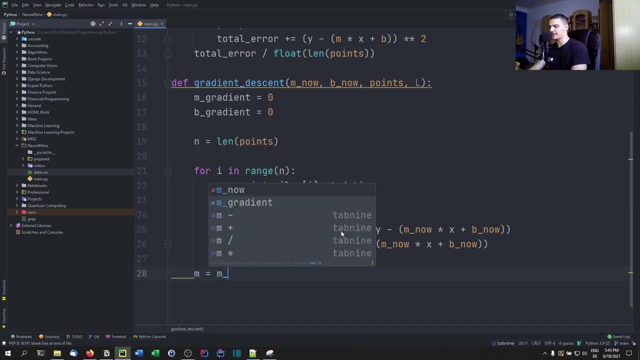 So we're just going to go back to the mathematical explanation. So we're just going to go back to the mathematical explanation. So what we do is we basically say, okay, the new m is going to be the m now, and we're going to say minus m gradient. so in the opposite direction, 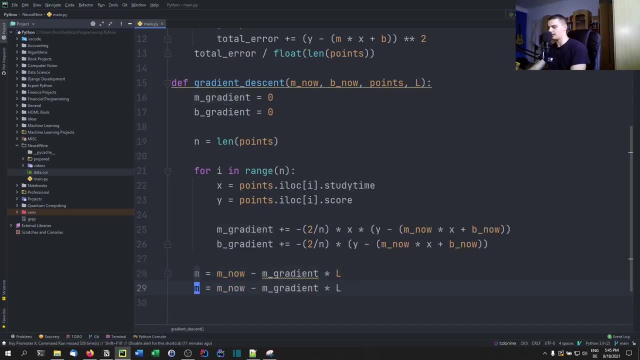 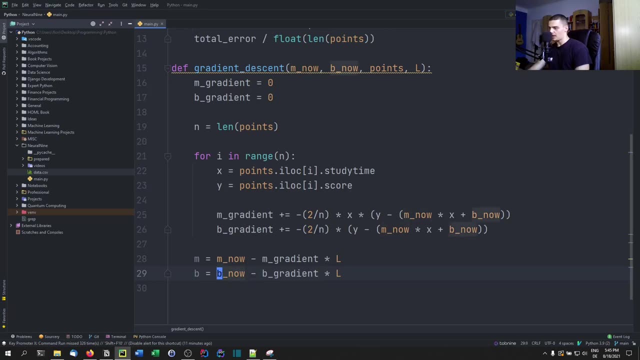 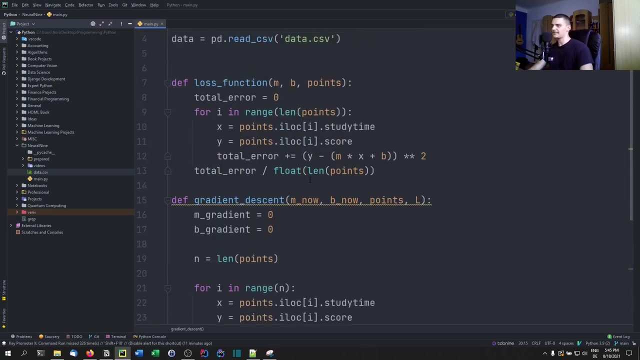 but with a learning rate of l That determines how much we move. Same for b, and that is actually it. And in the end, of course, we return m and b, both values. That is the gradient descent function. We can actually get rid of that function, if you're not. 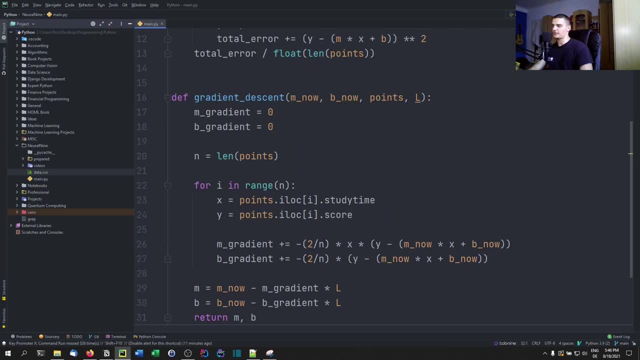 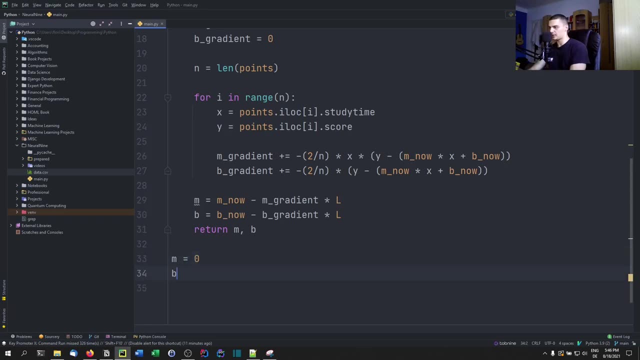 interested in it. but that is all we need to do in order to perform the linear regression. So now we just need to execute everything. We say, okay, what is m? We start with zero. B, we start with zero. We can pick any starting values if we want to. We will use a learning rate of 0.0001. 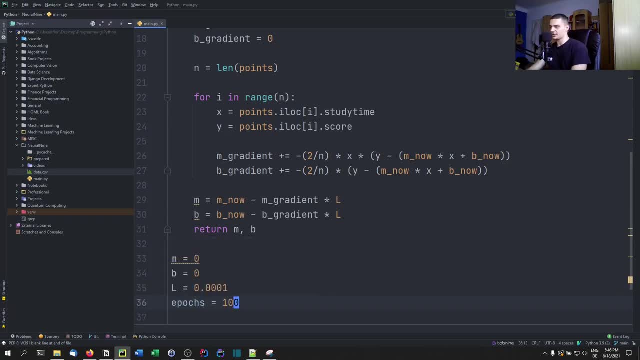 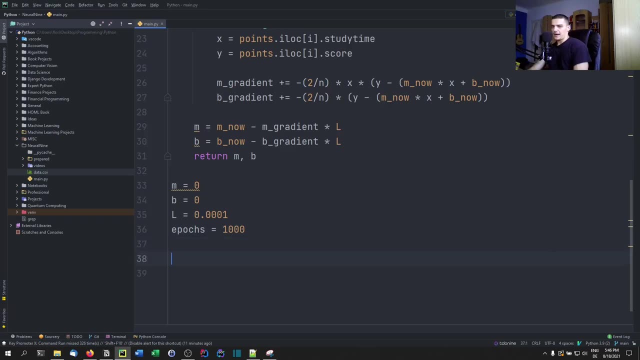 and we're going to use 100 iterations, also called epos. We can also go with 1000 actually, so let's go with 1000.. And now what we do is we just say, for i in range epos, So for the amount of iterations here. 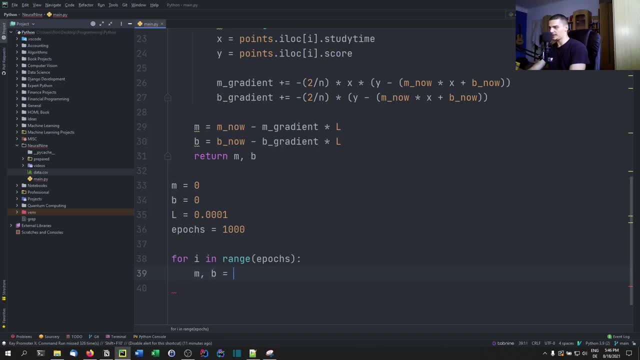 we're just going to say m and b are going to be gradient descent of m, b and the data and the learning rate. So we're constantly going to get better and better and better and better at estimating the perfect m and b And in the end 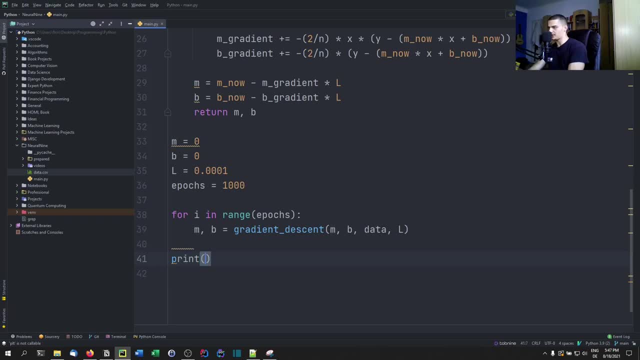 we can print PLT, we can print m and b And we can plot the results. So we can say: PLT dot scatter data dot study time, data dot score. color is going to be black, And then PLT dot plot And. 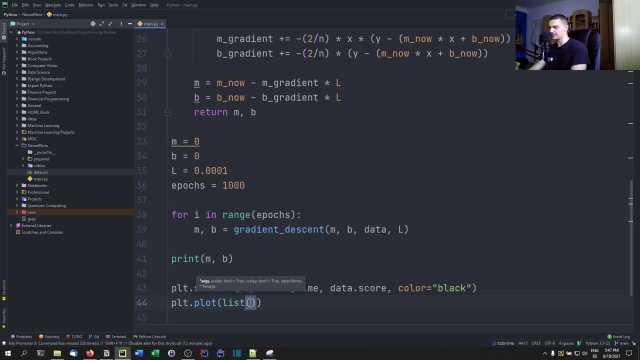 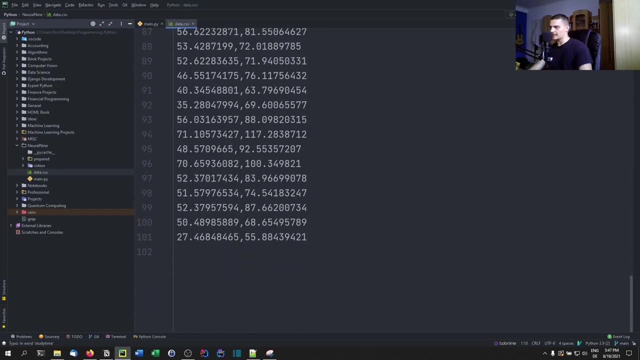 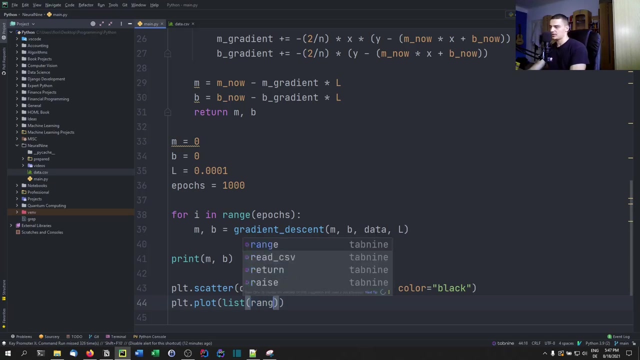 we can plot the trend line here, which is basically just a list, And we can look at the CSV file. all the values should be. all the x values at least should be more than 20 and less than 80. So we can just go with list range 20 to 80,.